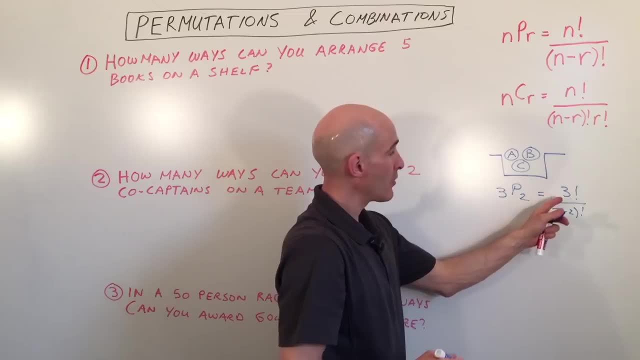 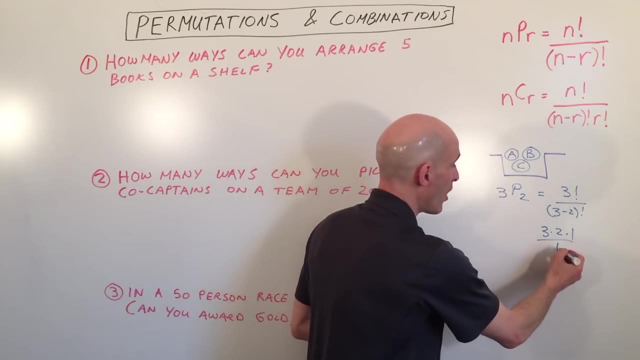 over three minus two factorial. Three factorial is just three times two times one. Three minus two is one factorial And you can see we have three times two, which is six. So if we want to write these down really quick, this is going to be A, B or you could get B and then A. That's considered. 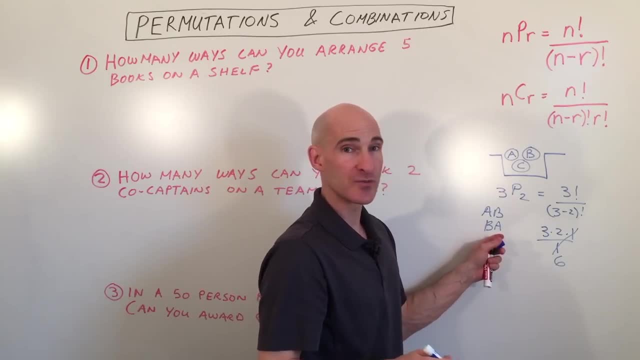 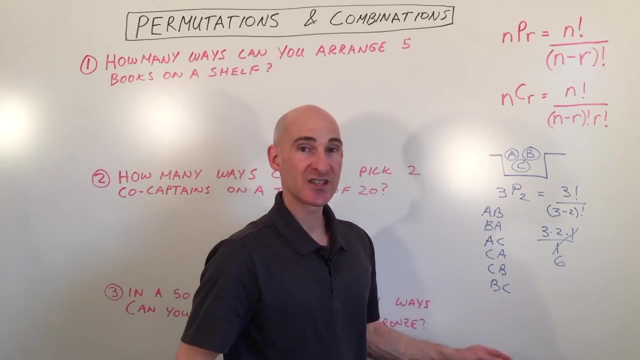 a different permutation, that's a different outcome, because order is important. You could get- let's see A, C, C, A and what else You could do- C, B, And you could also do B, b, c, So you can see there's six different ways to pick two marbles out of the three. 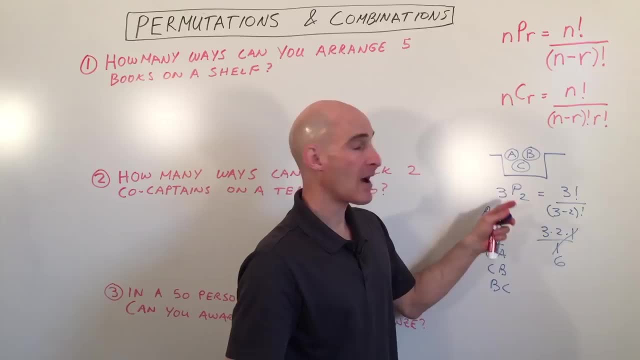 Now if we were doing combinations? okay, let's do the exact same problem. How many ways are there to choose two out of the three? Well, that's going to be three factorial over three minus two factorial, two factorial. Okay, so if we simplify this, we get three, two, one, Three. 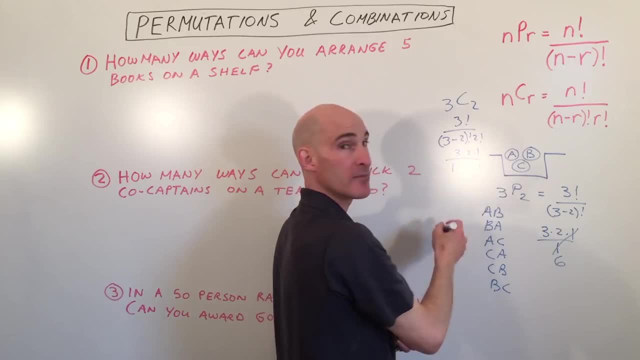 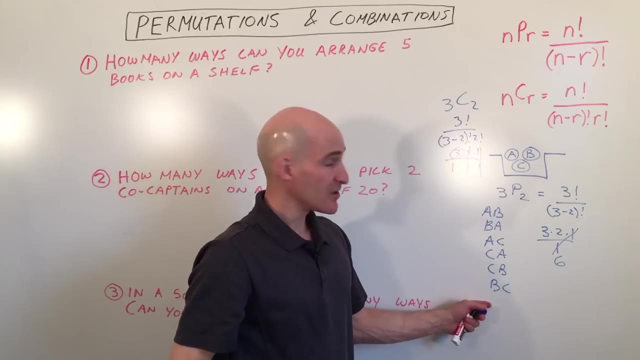 minus two is one factorial, which is one. Two factorial is two times one And you can see the twos, the ones, okay, and we're left with three divided by one, which is three. So let's go back to the outcomes here. Notice a, b and b? a from a combination perspective. those are the same two. 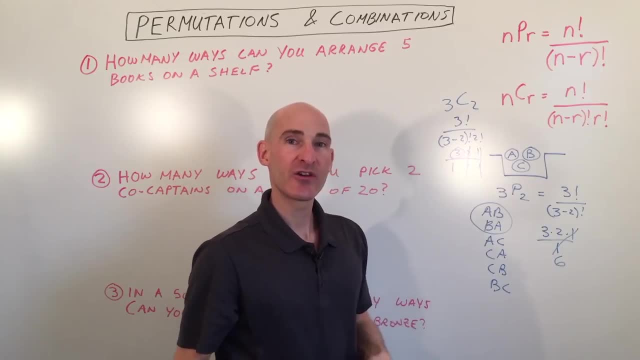 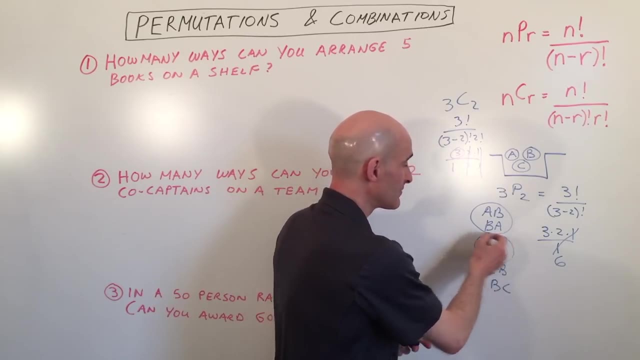 marbles. So whether you get a and b, b and a, you don't really care. You say, well, I've got the same two marbles right. So that's just one outcome Here. we've got a and c, c and a- Those 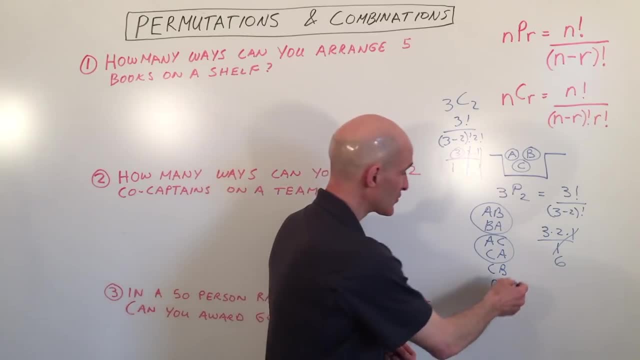 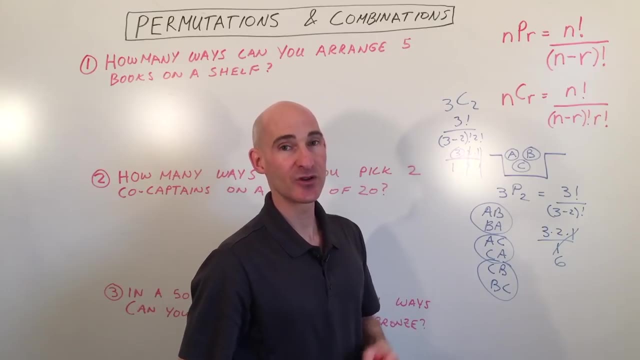 are the same two marbles, And c and b, b and c, those are the same two marbles. So you can see, when you're doing combinations, where the order doesn't matter, you're going to have fewer possibilities, fewer outcomes. And you can see here in the formula this: r, factorial, okay, here, in this case two. 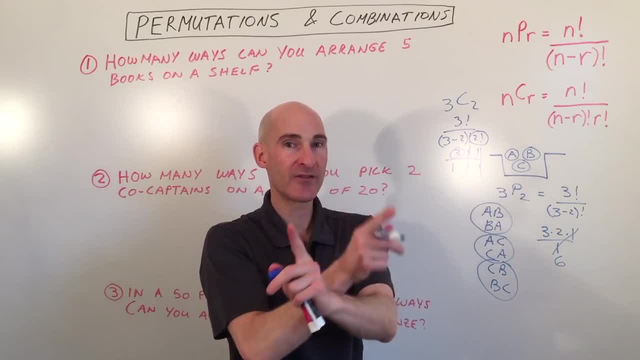 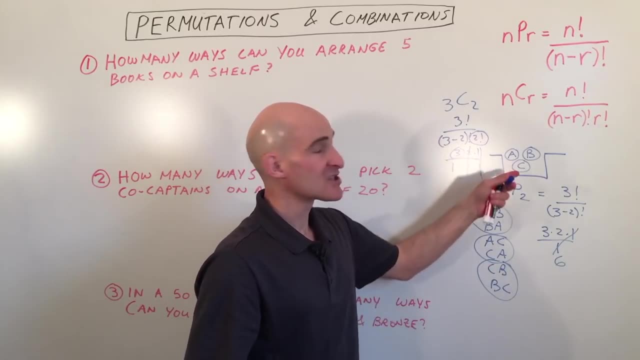 factorial what you're doing, because there's two items and you can have them two different ways. you're dividing out those duplicates, okay, or those multiplicities. So this is just a simple example. Let's get into some other examples. Let's do this one here. How many ways? 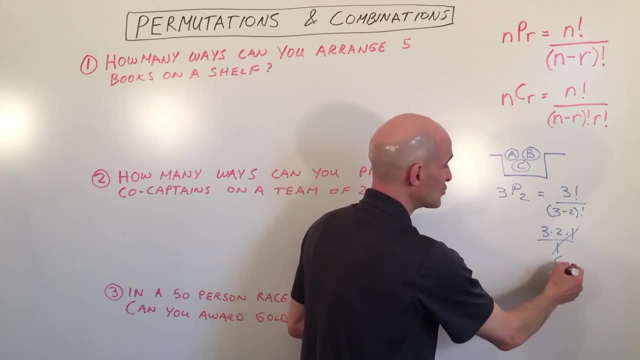 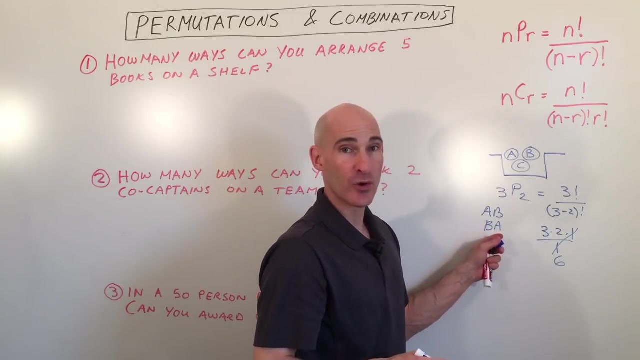 which is just one, and you can see we have three times two, which is six. So if we want to write these down really quick, this is going to be a, b or you could get b and then a. That's considered a different permutation, That's a different outcome, because order is important. You could get: 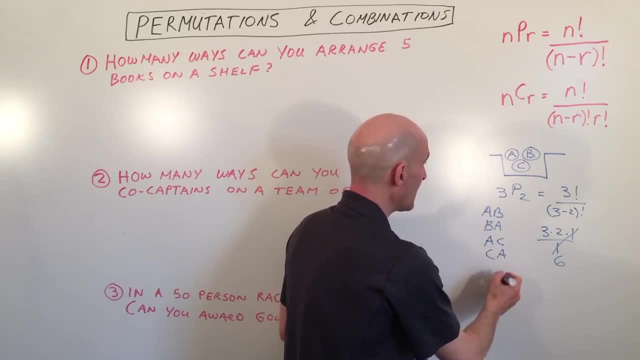 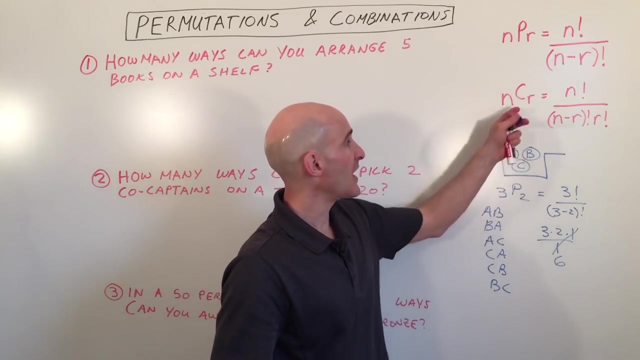 let's see a, c, c, a And what else You could do: c, b, and you could also do b, c, So you can see there's six different ways to pick two marbles out of the three. Now, if we were doing combinations, Okay, let's do the. 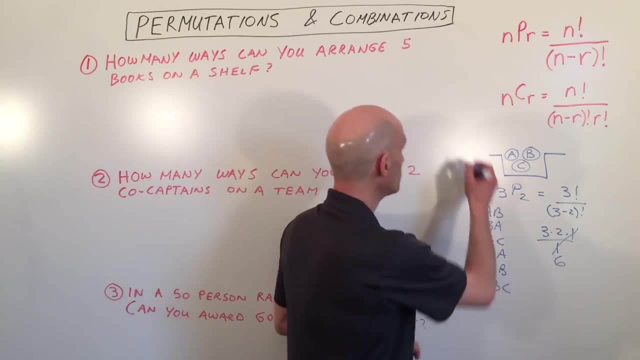 exact same problem. How many ways are there to choose two out of the three? Well, that's going to be three factorial over three, minus two factorial, two factorial. Okay, so we're going to do a permutation. So we're going to do a permutation. So we're going to 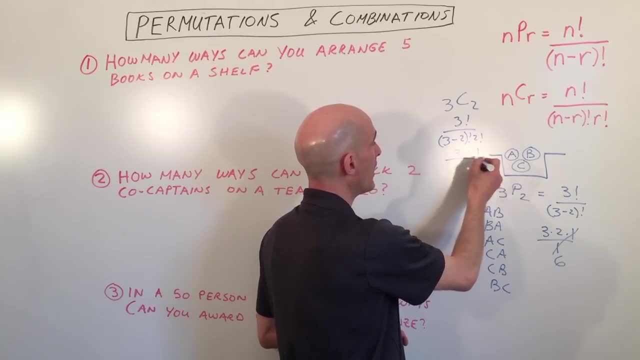 simplify this, Okay. so if we simplify this, we get three, two, one. Three minus two is one factorial, which is one. Two factorial is two times one, And you can see the twos, the ones, Okay, and we're left with three divided by one, which is three. So let's go back to the outcomes here. Notice a, b and b a. 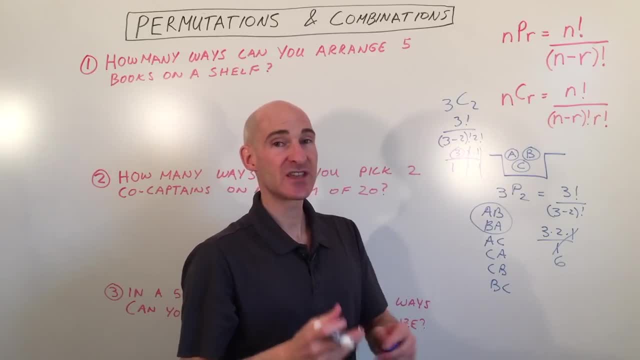 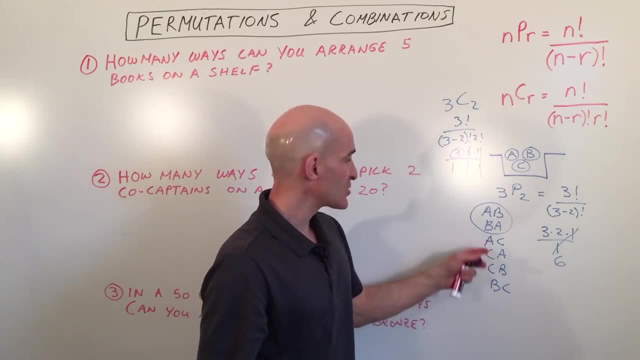 from a combination perspective, those are the same two marbles. So whether you get a and b, b and a, you don't really care. You say, well, I've got the same two marbles right. So that's just one, one outcome. Here we've got a and c, c and a. Those are the same two marbles, And c and b, b and c, Those are the same. 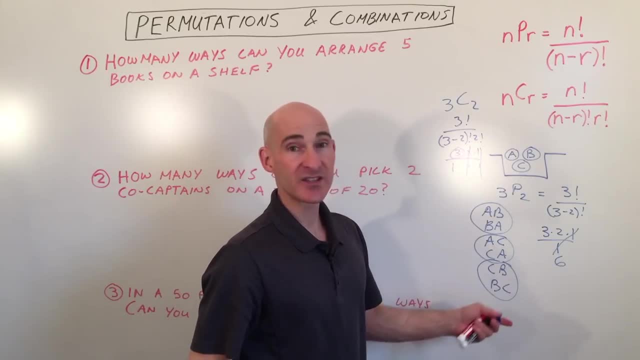 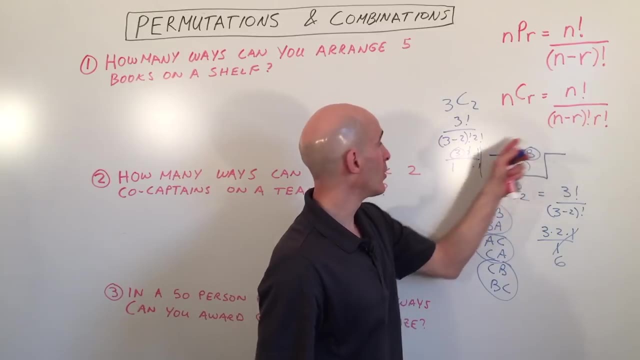 two marbles. So you can see when you're doing combinations where the order doesn't matter, you're going to have fewer possibilities, fewer outcomes. And you can see here in the formula this: r factorial- Okay, here, in this case, two factorial What you're doing, because there's 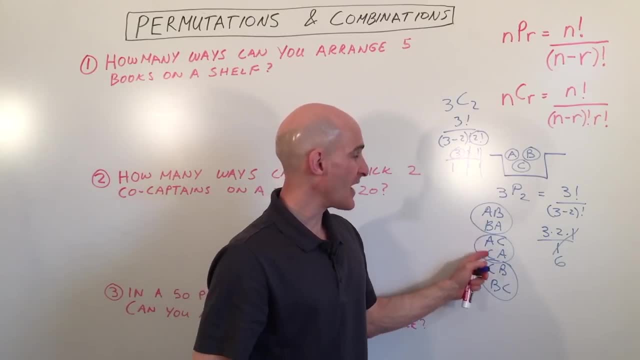 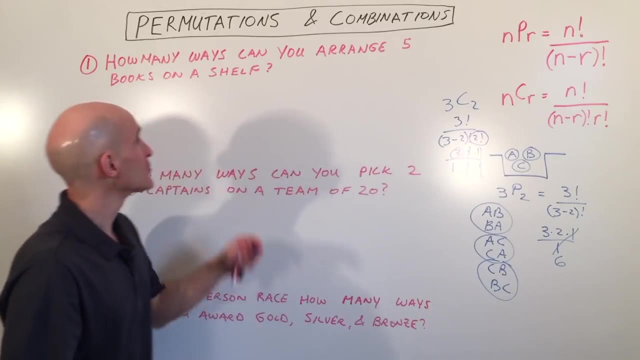 two items and you can have them two different ways. You're dividing out those duplicates, Okay, or those multiplicities. So this is just a simple example. Let's get into some other examples. Let's do this one here: How many ways can you arrange five books? 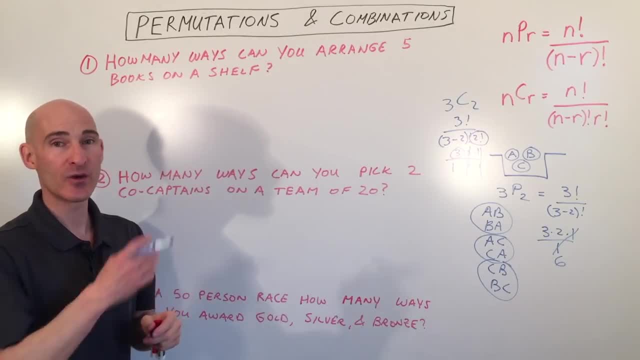 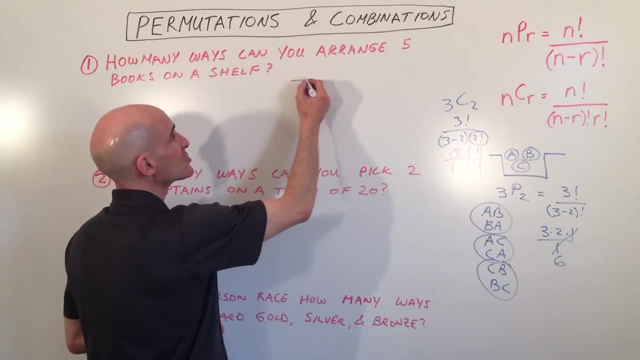 can you arrange five books on a shelf? okay, where the order is important. So you want to put the books like that. Well, there's a couple different ways to do this problem. One way to do it is just to diagram it out like this And you can say: well, there's five choices for the book. 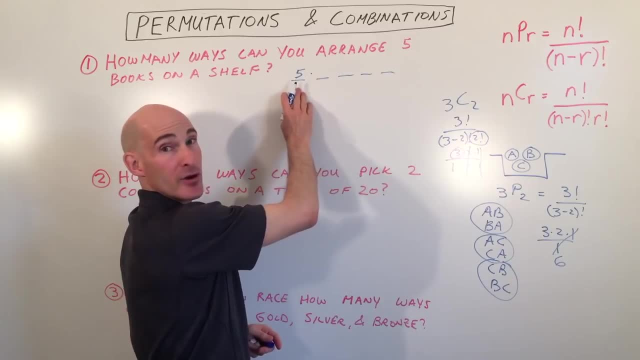 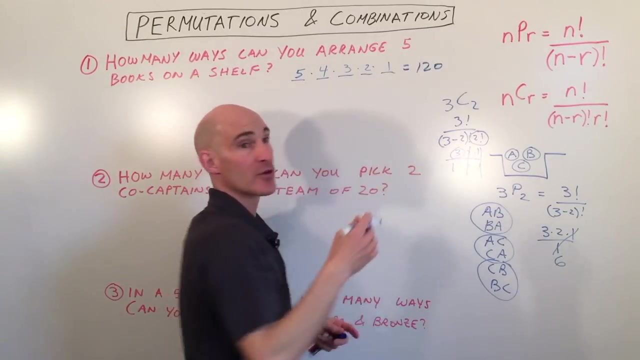 that I put here right. Then, once I put that book there, there's only four books left from which to pick from, to put in the second position, And then it goes down from there: three, two, one, And if you do that, you get 120 different permutations, different orderings, right? The other way to do. 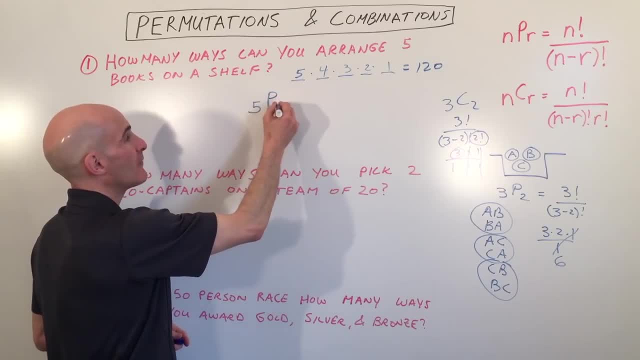 this problem is: you could say: well, out of five books, how many ways can I pick five? Okay, the P stands for permutations, but I just like to say pick five. So, out of five total, how many ways can you pick five? where the order matters. So if we go to our formula here, the NPR formula, we have 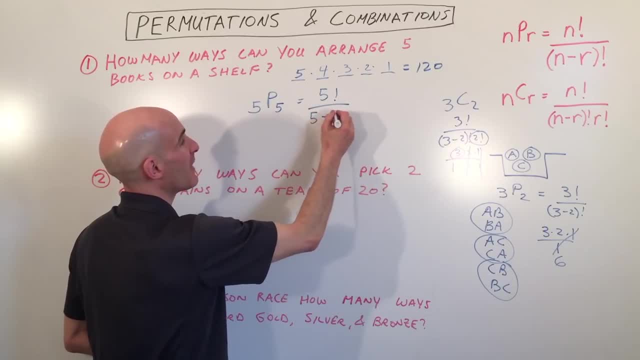 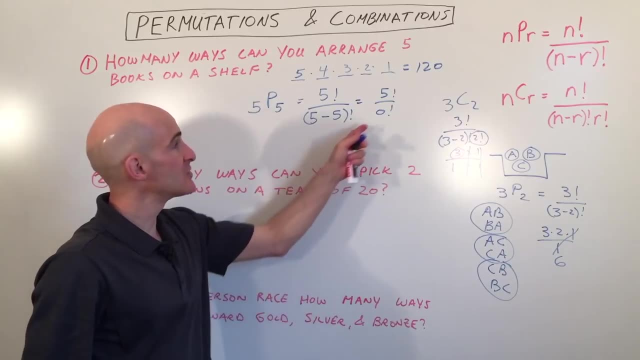 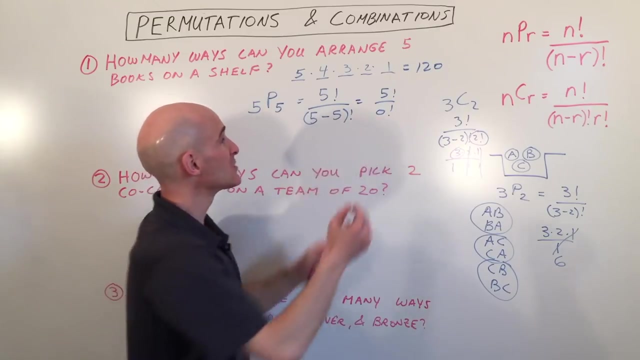 five factorial over five minus five factorial, That's five factorial over zero factorial. And remember: zero factorial actually equals one. That's just something you'll have to memorize. One factorial is one and zero factorial is one, So this just ends up being: 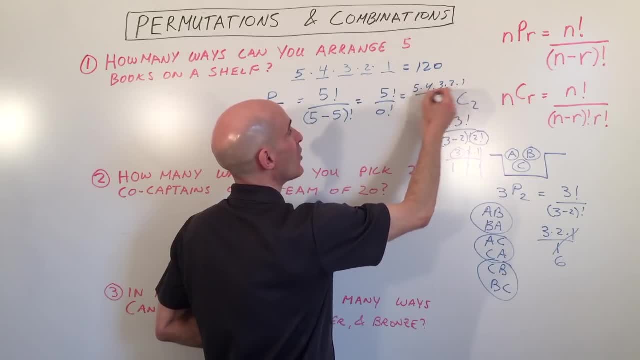 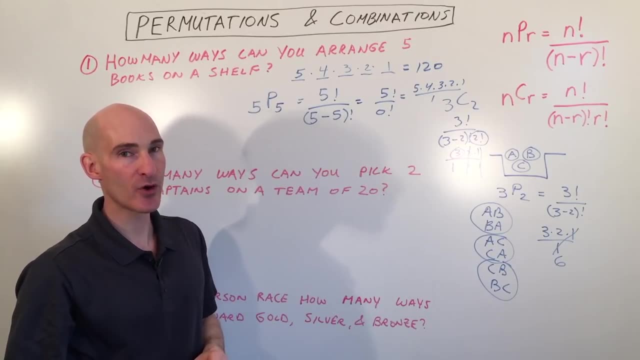 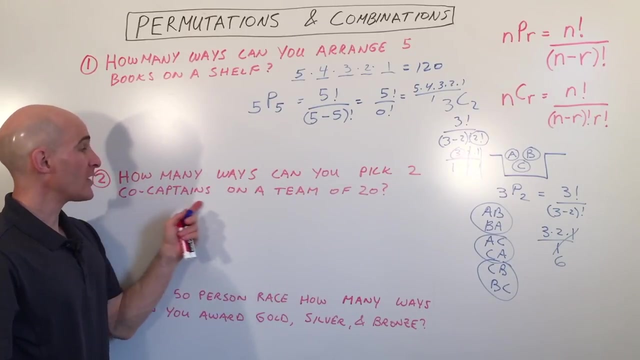 five times four times three times two times one, all divided by one, which is the same thing, we got here 120.. So you can see, sometimes there's a couple different ways to approach these problems. Let's look at the next one. How many ways can you pick two co-captains? 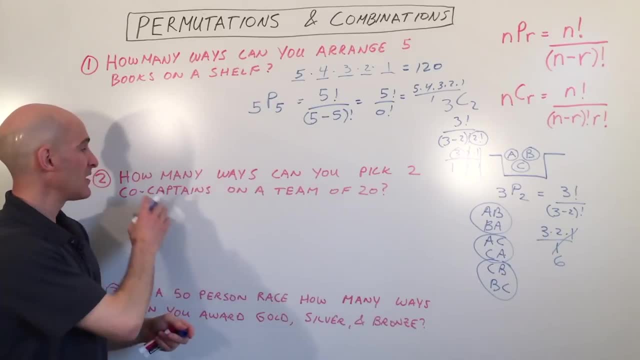 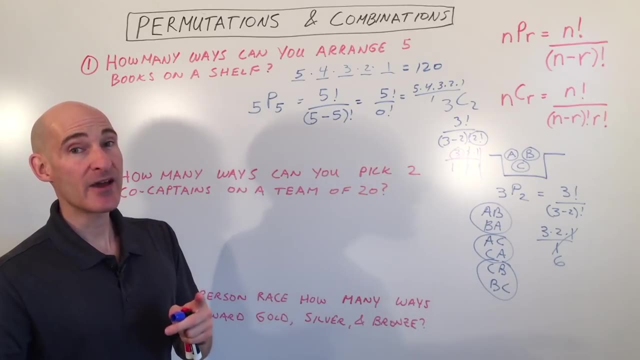 on a team. There's a team of 20.. So visualize you're on a sports team, There's 20 players and you want to pick two co-captains. Now let me ask you a question: Does the order matter? Is there like a head co-captain? 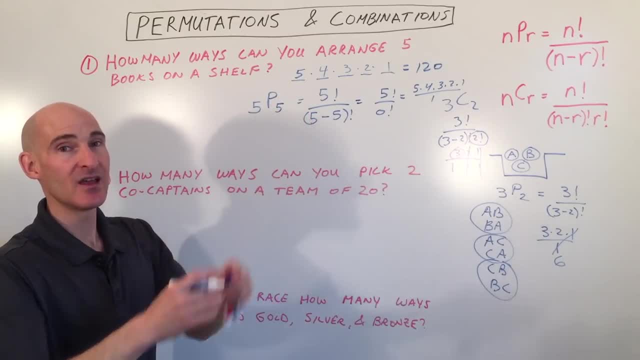 Like a assistant co-captain, Or are they the same? In this case, they're the same. It doesn't specify any importance as far as the order is concerned. So that tells us that we're going to be using which one- Permutations or combinations, Combinations- because the order doesn't matter. So what we're? 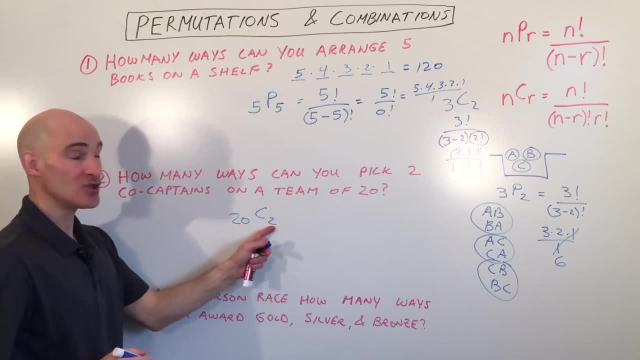 going to do is, out of five books, we're going to pick two co-captains. So that tells us that we're going to have 20 players. We're going to choose two, Okay, so this is a total. We're choosing two. Let's use. 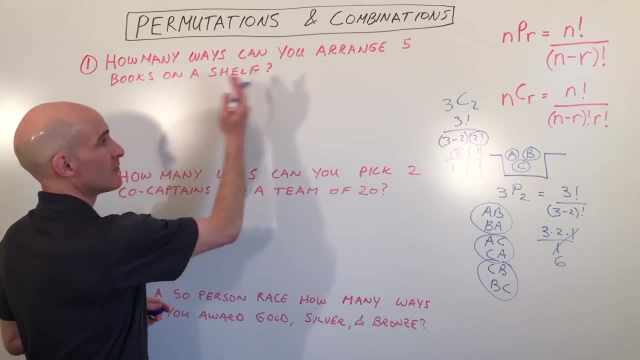 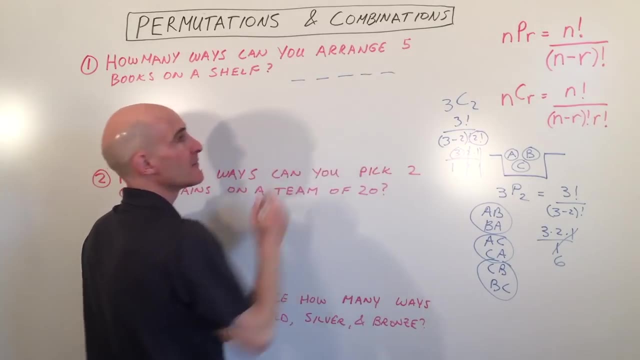 on a shelf, Okay, where the order is important. So you want to put the books like that. Well, there's a couple different ways to do this problem. One way to do it is just to diagram it out like this And you can say: well, there's five choices for the book that I put here, Right. Then, once I put that book, 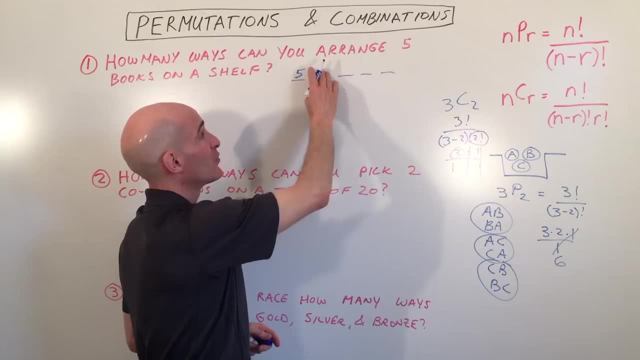 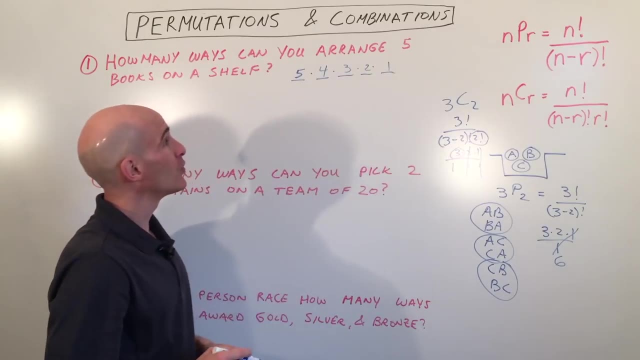 there there's only four books left from which to pick from to put in the second position, And then three, two, one, And if we multiply all those together we get 120 different permutations, different orderings, Right. The other way to do this problem is you can say: well, out of five books. 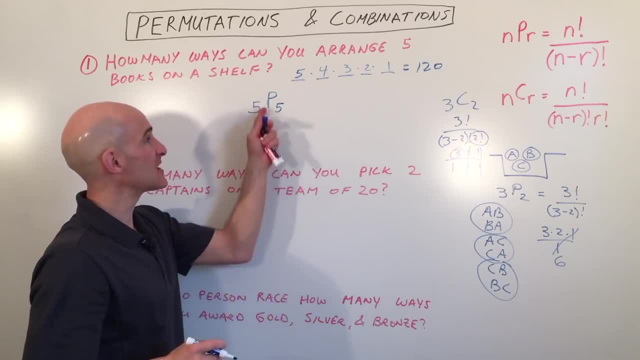 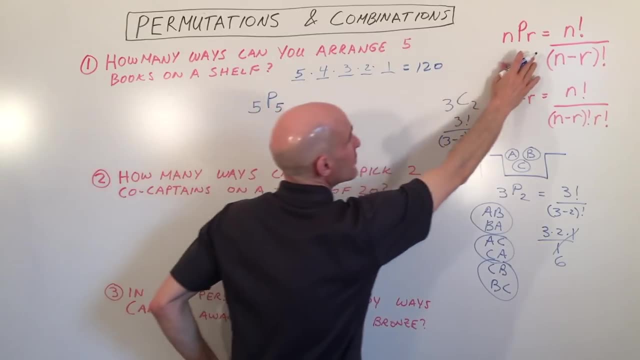 how many ways can I pick five? Okay, the P stands for permutations, but I just like to say pick five. So, out of five total, how many ways can you pick five? where the order matters? So if we go to our formula here, the NPR formula, we have five factorial over five factorial, So five factorial over five factorial. 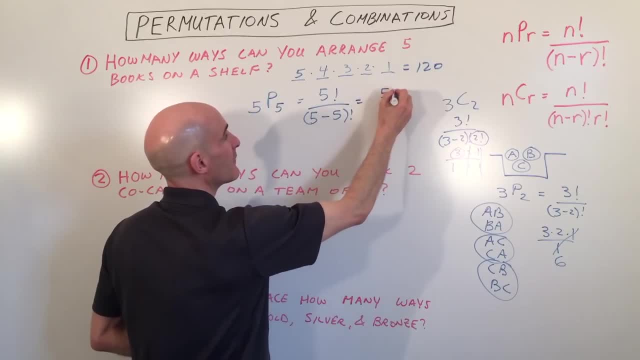 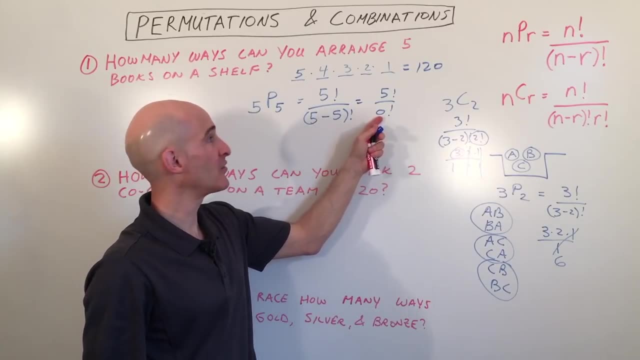 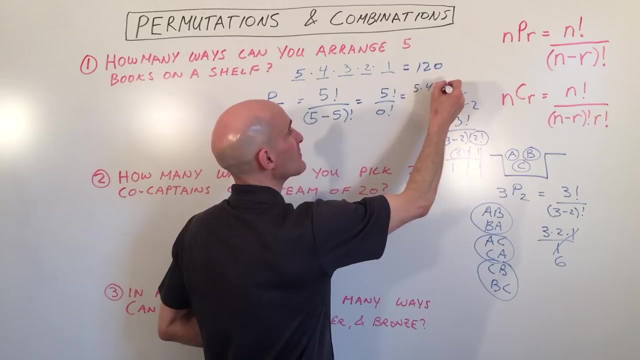 That's five factorial over zero factorial. And remember, zero factorial actually equals one. That's just something you'll have to memorize. One factorial is one and zero factorial is one. So this just ends up being five times four times three times two times one, all divided by one, Which is the same. 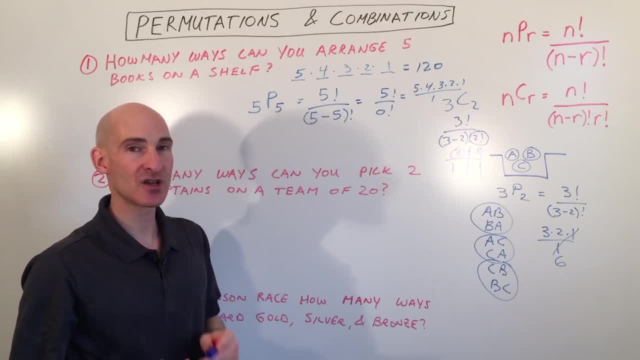 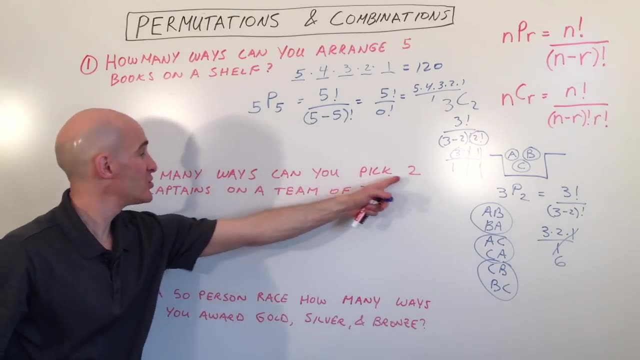 thing we got here 120.. So you can see, sometimes there's a couple different ways to approach these problems. Let's look at the next one. How many ways can you pick two co-captains on a team of 20.. So visualize you're on a sports team. 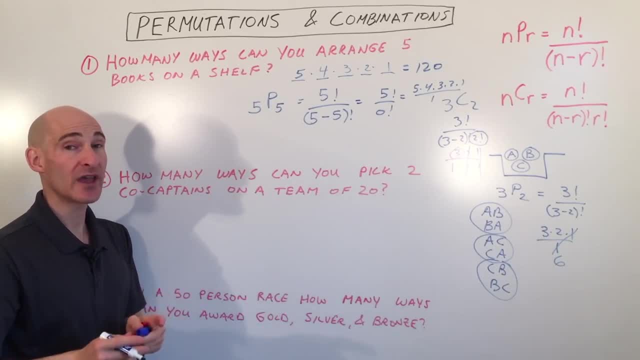 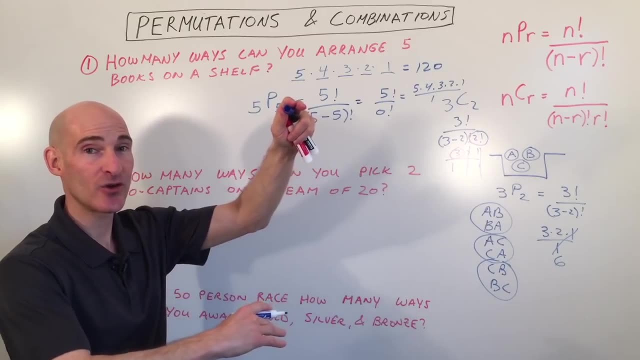 There's 20 players and you want to pick two co-captains. Now let me ask you a question: Does the order matter? Is there like a head co-captain, like a assistant co-captain, or are they the same? 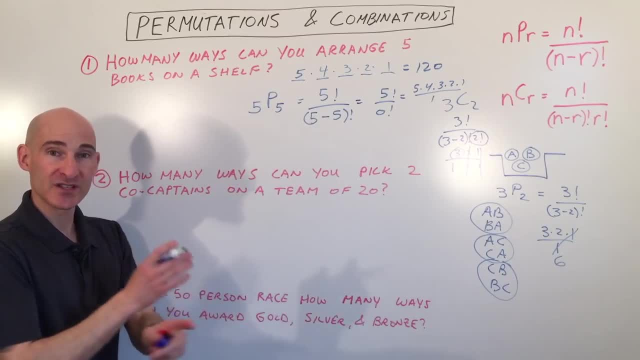 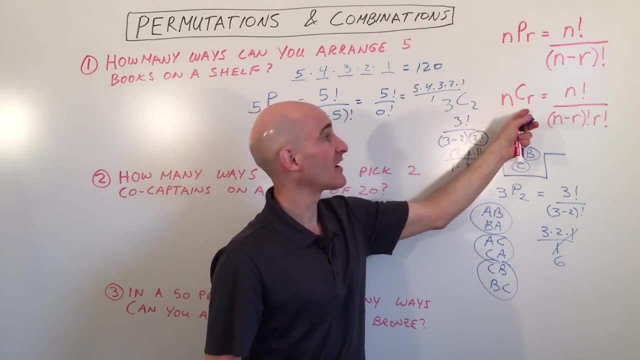 In this case they're the same. It doesn't specify any importance as far as the order is concerned. So that tells us that we're going to be using which one permutations or combination Combinations, because the order doesn't matter. So what we're going to do is, out of 20 players, we're.